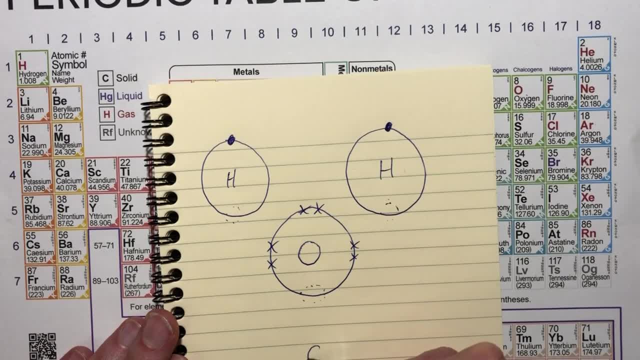 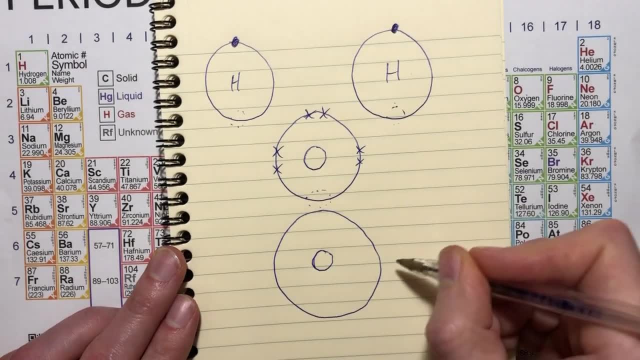 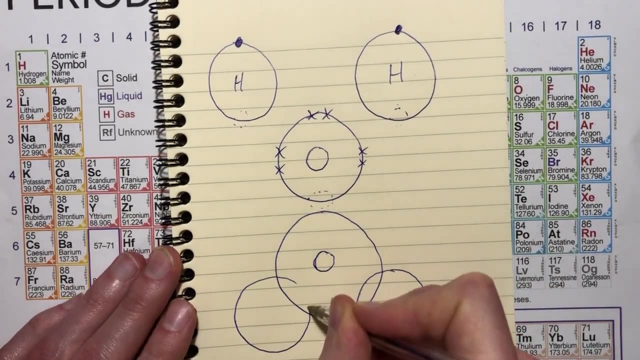 So what's going to happen? We're going to draw this like this: We're going to repeat the oxygen atom down here and I'm going to overlap it with the hydrogens. So the hydrogen electrons are now going to overlap Like this: 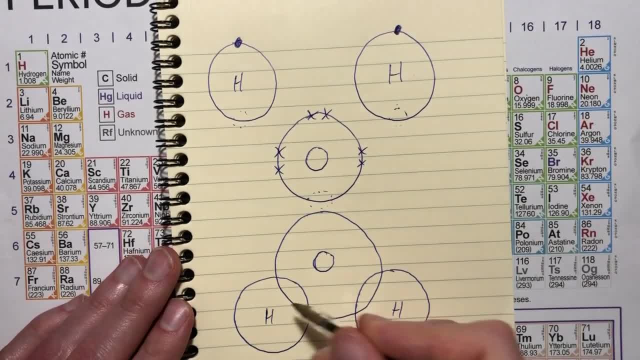 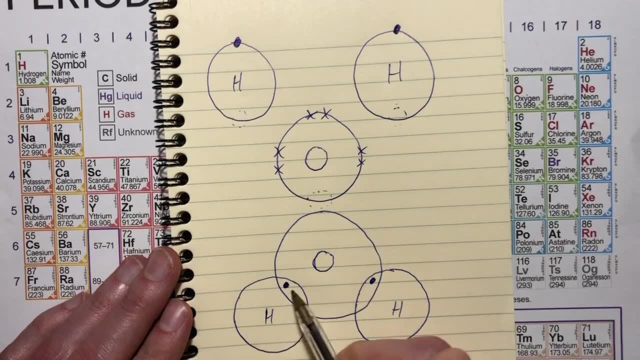 And when they do, this shows that they're sharing their electrons. So hydrogen's electron now goes in the gap here and here, And that means that this electron is actually orbiting both the hydrogen and the oxygen, And that's what a covalent bond is. 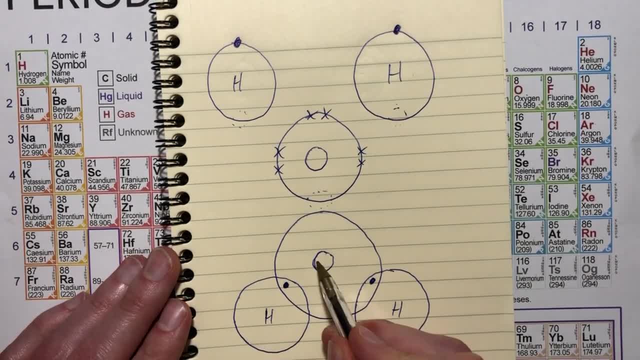 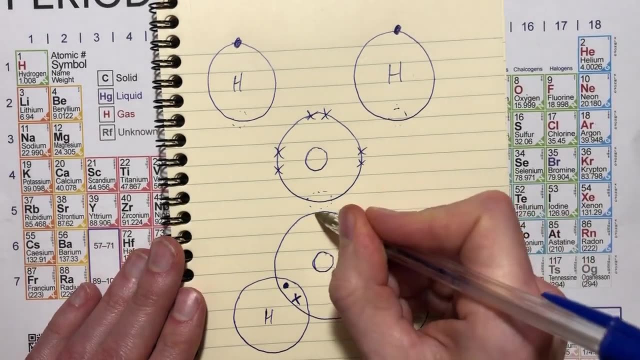 But they agree to share them. So if hydrogen is giving oxygen its electron, it expects one in return. So oxygen donates an electron there And the same thing happens here. So that's two crosses, but there were six originally, So we need to put them back in as well. 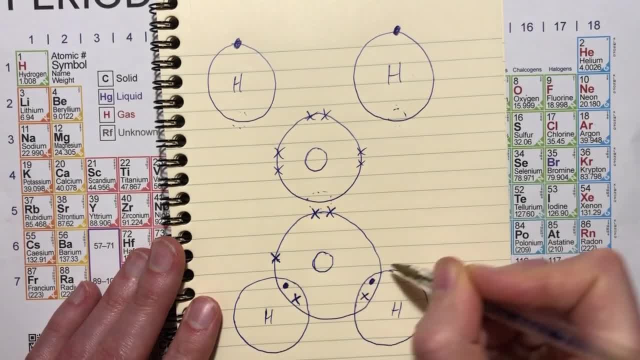 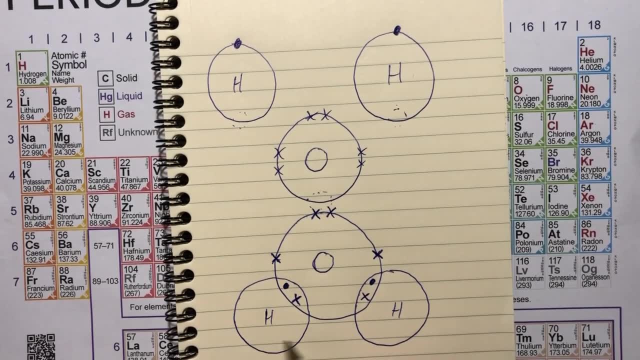 So that's now four electrons, five and six, And now if we count up, we can see that hydrogen has two electrons in its shell, So it's happy because it's the first shell, so it only needs two. Another two there.